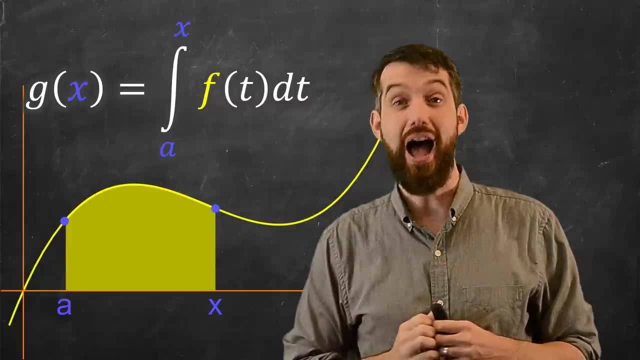 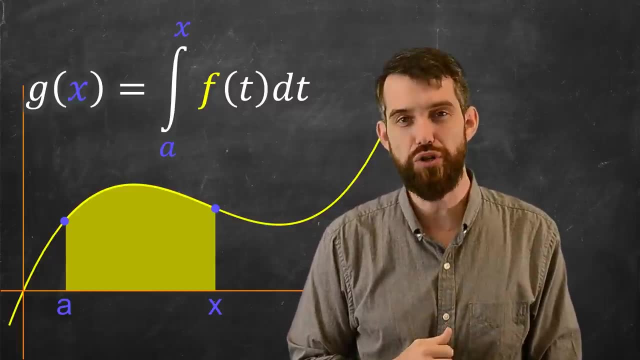 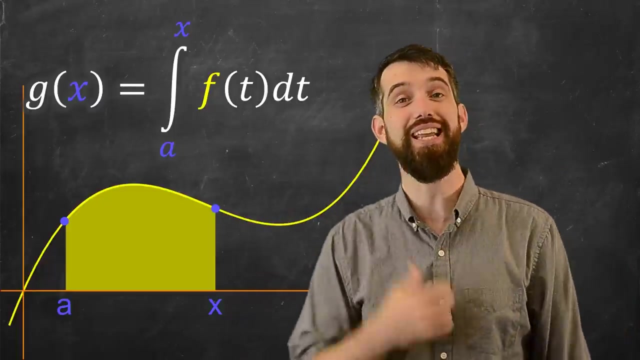 of x. One thing to note here is that in this particular curve I've managed to draw one which is a positive function. This function of x is over the x-axis. So as I go to the right, as x is increasing, the area is also increasing. So this g of x here is an increasing 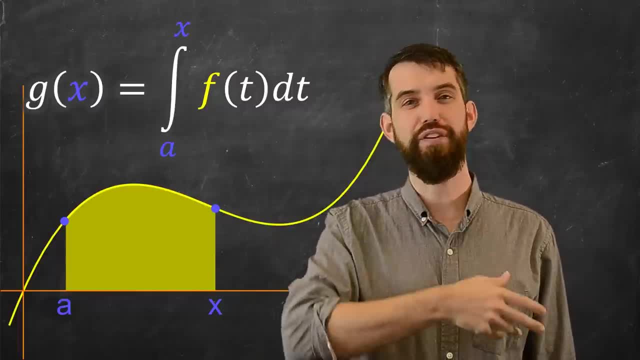 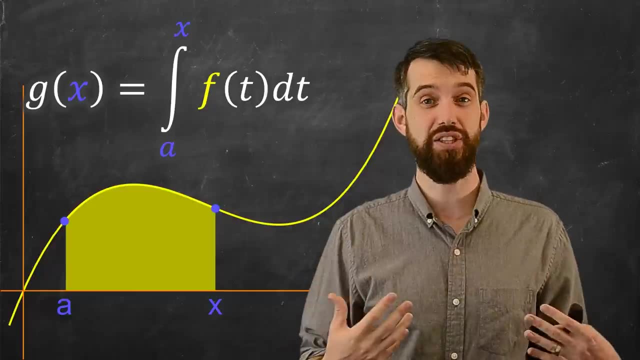 function as long as f is positive. If in a different graph, the function dipped beneath the x-axis and was negative at some point, then the g of x, the accumulation function, would start decreasing at the point as I was adding negative areas. contributions from: 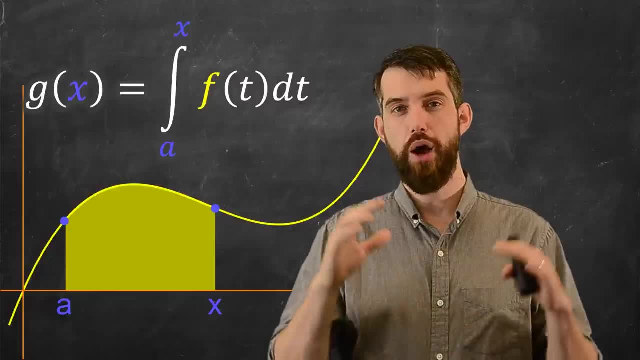 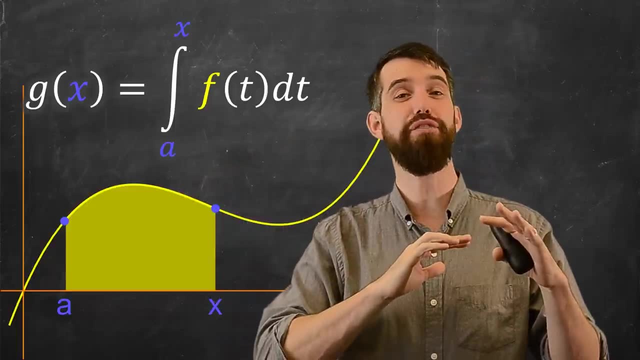 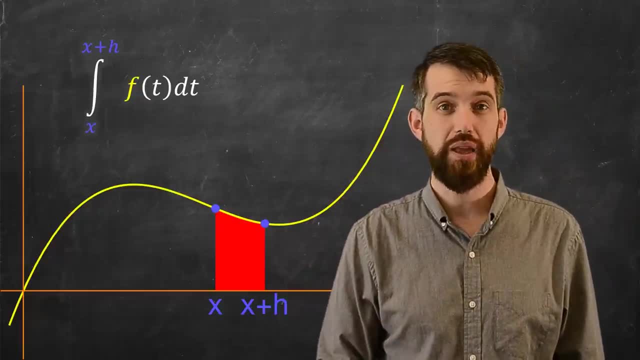 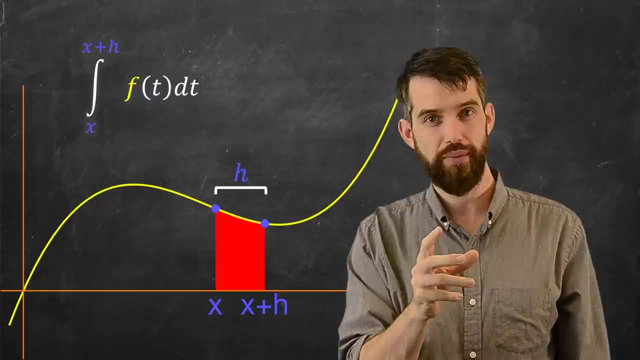 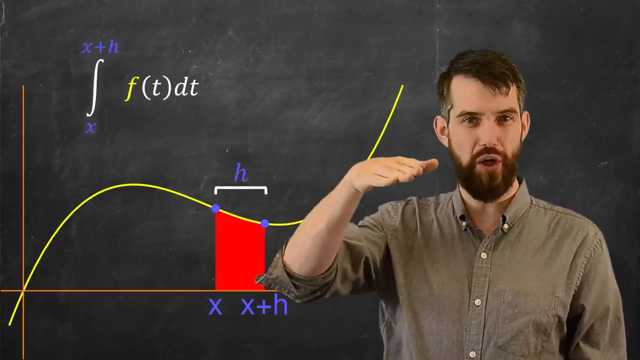 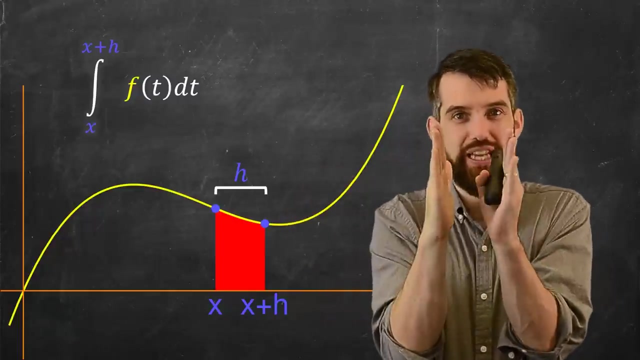 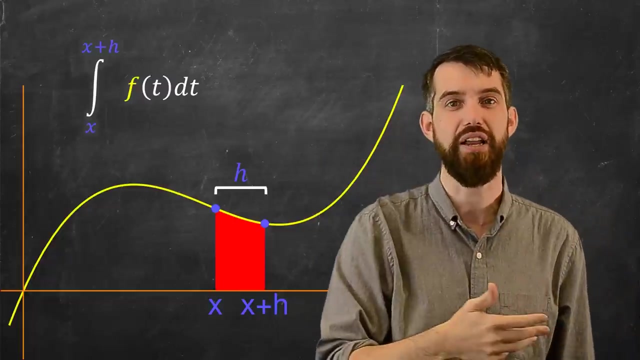 What looks like a rectangle and, I think, some weird curve along the top. However, imagine that my x was really really small, so my x and my x together are right beside each other. Well, you could also approximate rectangle with a fixed height, That is, we could say that this was the rectangle that had the width. 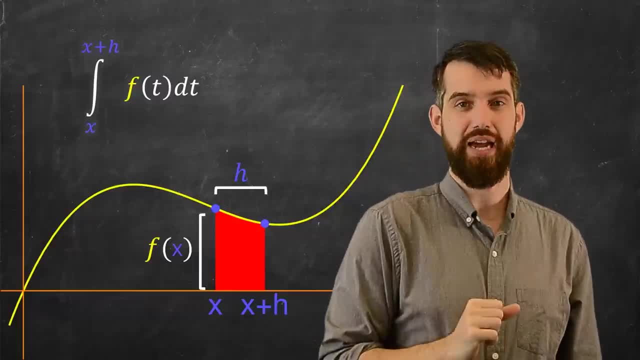 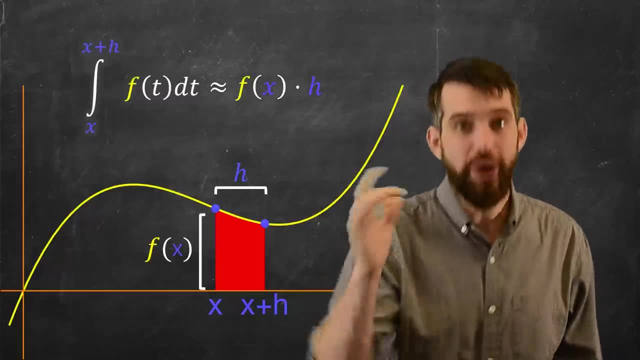 h but had a height of about f of x, And you might say, well, hold on, no, it's not quite a rectangle, But as my h goes to zero, this is approximately a rectangle of width h and of height f of x. 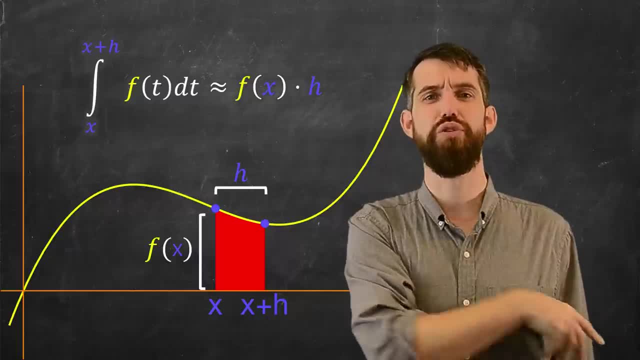 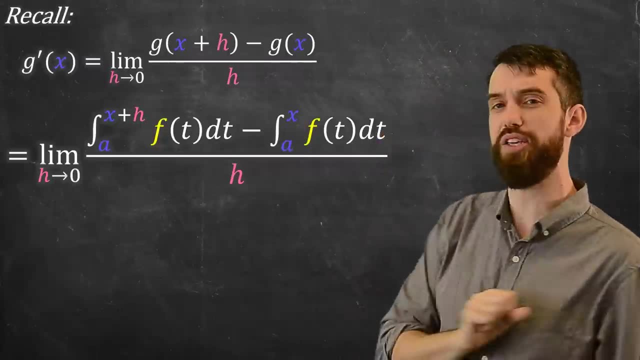 Let's take this result and let's put it back into my definition of the derivative, the definition for g prime of x. So this is where I was at earlier. I had my g prime, I did my definition of the derivative, I plugged in my accumulation functions. but now I can do something with that. 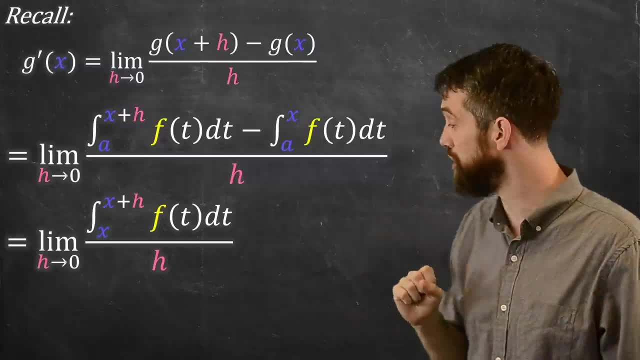 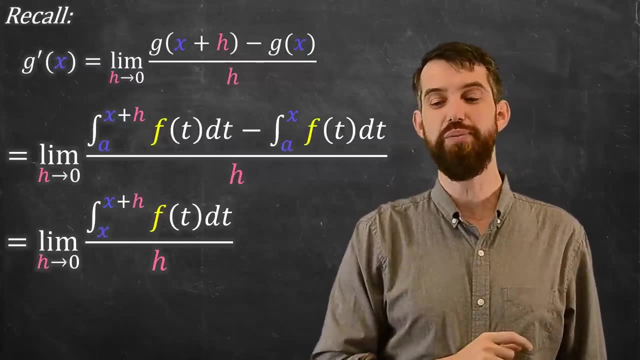 numerator. I know what that is. My approximation was that that numerator was just going to be the same thing as the integral from x up to x plus h of f of t, dt, and that was approximately just going to be f of x times h. And then I'm just about done with my proof here, because I got an h. 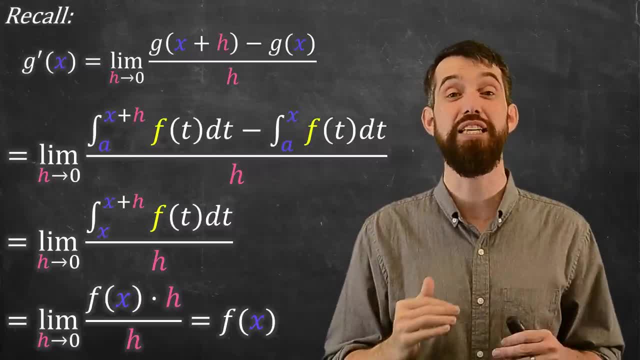 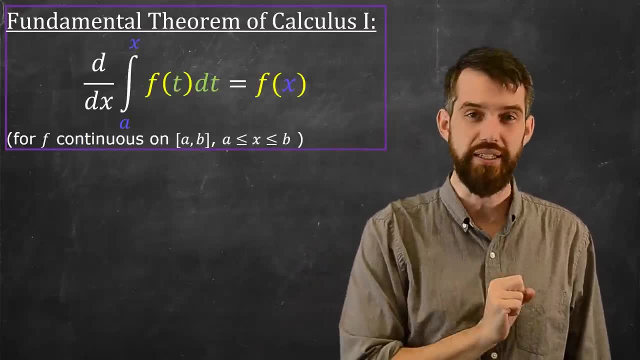 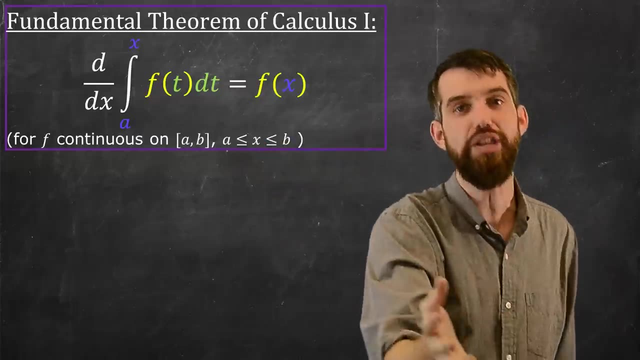 on the top, I got an h on the bottom. I can cancel those and that just leaves me with f of x. So the grand statement of the fundamental theorem of calculus number one is that the derivative with respect to x- my g prime here- the derivative with respect to x- of the accumulation function. 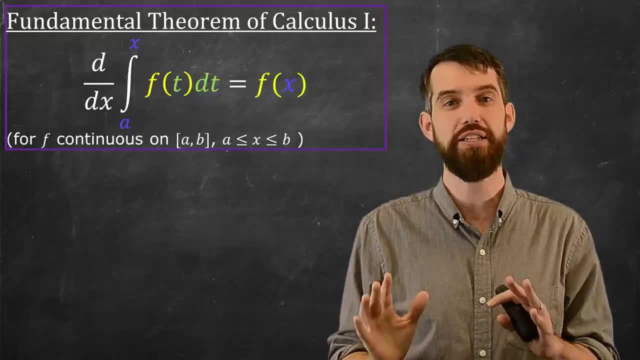 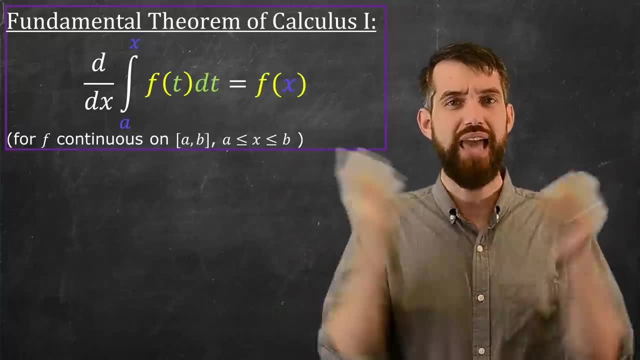 the integral from a up to x of f of t, dt is just f of x, And doesn't it sort of look here like derivatives and integrals cancel them. Indeed, we've got a derivative and an integral, and it does cancel. Now we have to be a little bit precise about what we mean by that, but we have. 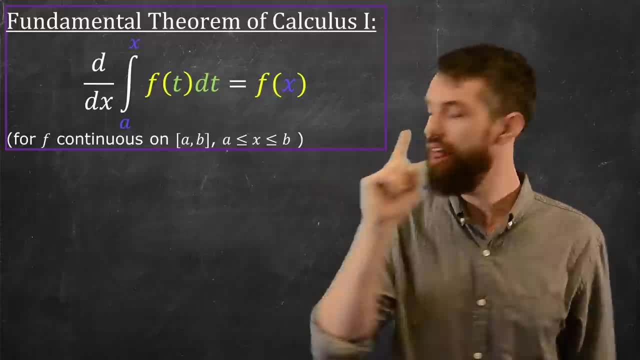 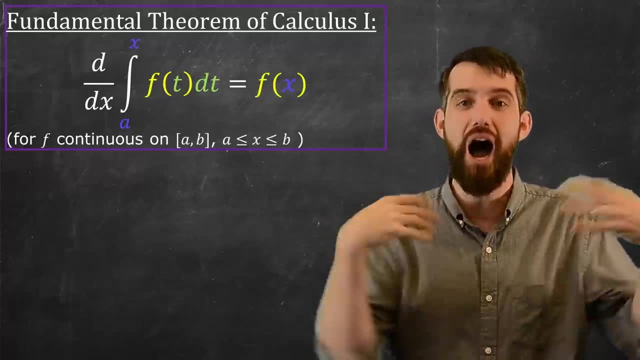 to be a little bit precise about what we mean by that. What we mean is exactly this statement. Note, by the way, that the t, that dummy variable that we have here. it becomes an f of x at the end. so this is a function of x, so the final answer should be f of x. it shouldn't be f of t the dummy. 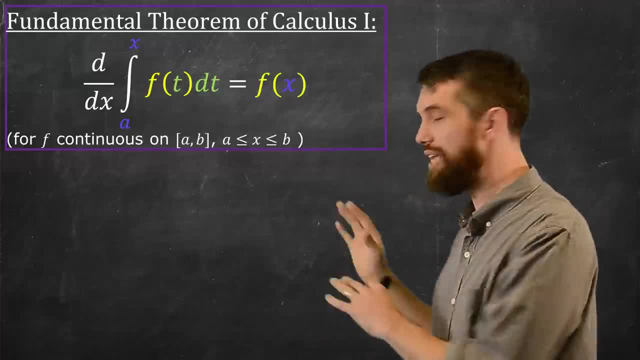 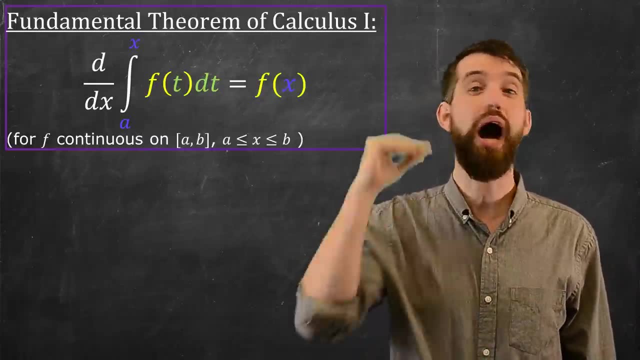 variable- And also note that this is very precisely needing to be written- the derivative not just of any integral, but precisely the derivative of the integral from a value up to x of some particular integrand in terms of t. So that's the end of the theorem and I'm going to end it here. 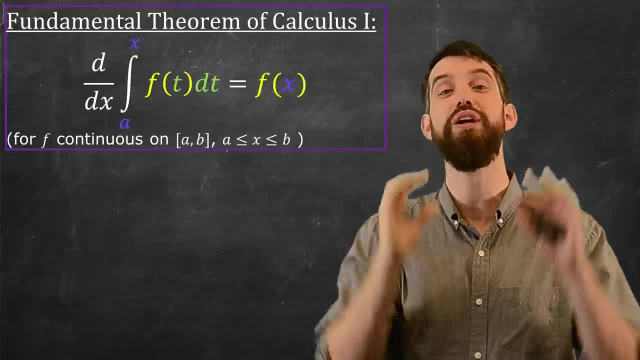 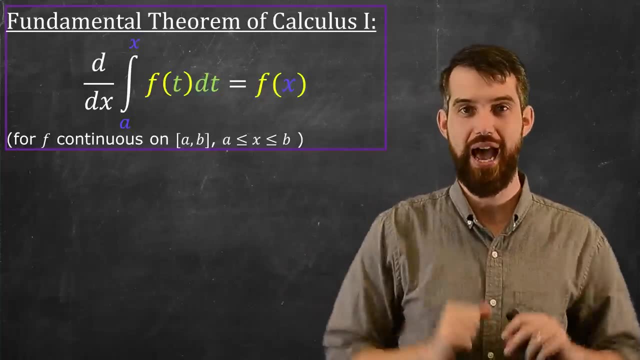 That is the fundamental theorem of calculus. It does have an assumption it has that this original function f needs to be continuous on a up to b, where x is some value in between a and b. but there you have it. Finally, let's go and use this theorem for something. I've got an example. it's kind. 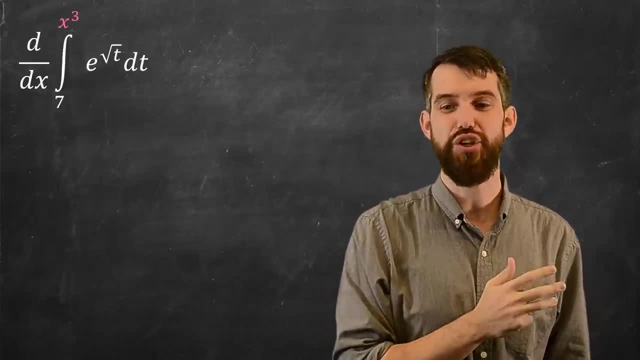 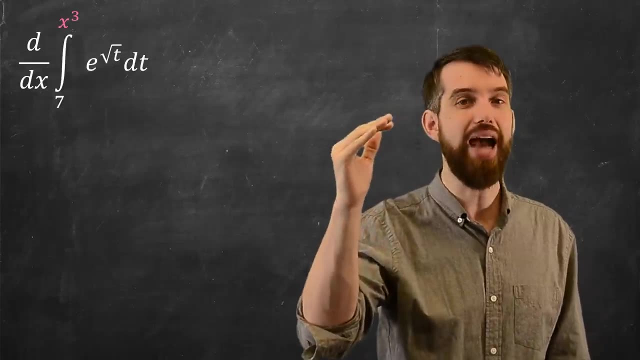 of a bit of a weird example, but we're going to apply it. So let's imagine that what my goal now is to be doing: the derivative with respect to x of the integral from 7, not up to x, but 7 up to x cubed. 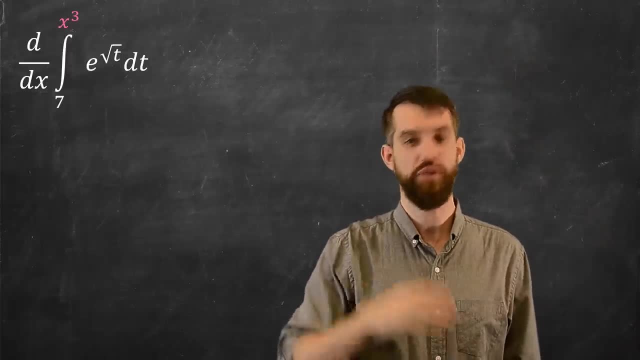 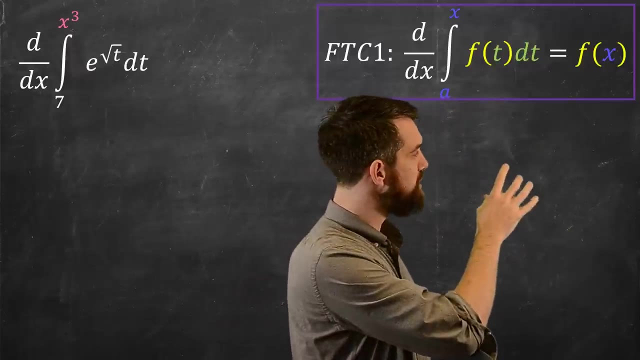 of e to the square root, t, dt. And, of course, I'll remind yourselves that the fundamental theorem of calculus is what we have right here, the derivative of these things. but notice, the fundamental theorem of calculus only goes from a all the way up to x. Well, how can I deal with this? Because 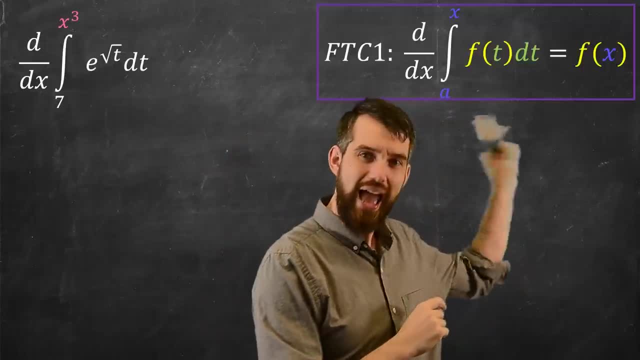 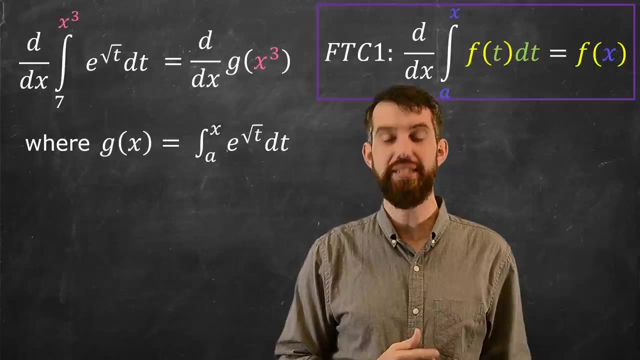 I've got an x cubed in my example, but I only have an x in the statement of my theorem. The trick is going to be chain rule. So what I'm going to do is say that this thing here, this particular derivative, is derivative of some function of x cubed, and I'm going to say that this thing here 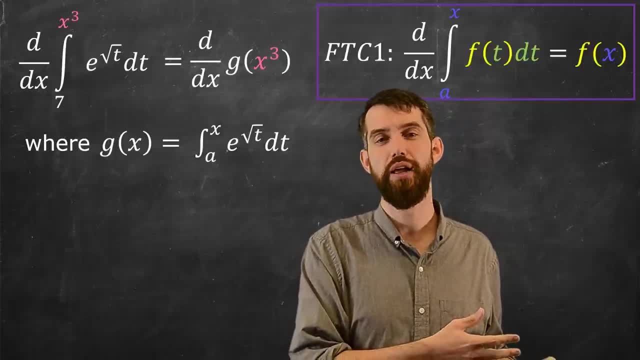 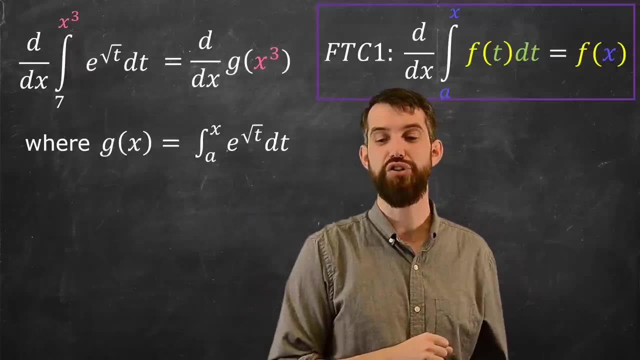 is derivative of some function g, the accumulation function we saw earlier, but that accumulation function composed with the function x cubed. So g of x is the accumulation function and g of x cubed is that same accumulation function where every time there's an x because of the composition. 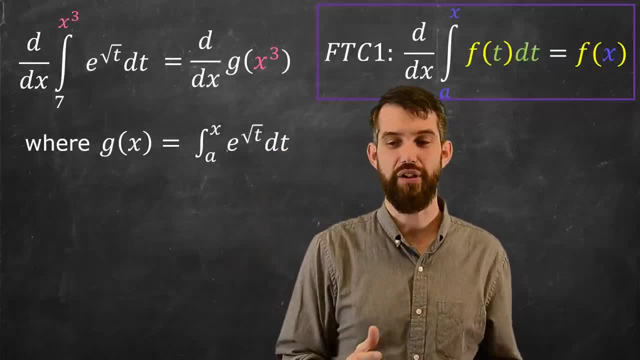 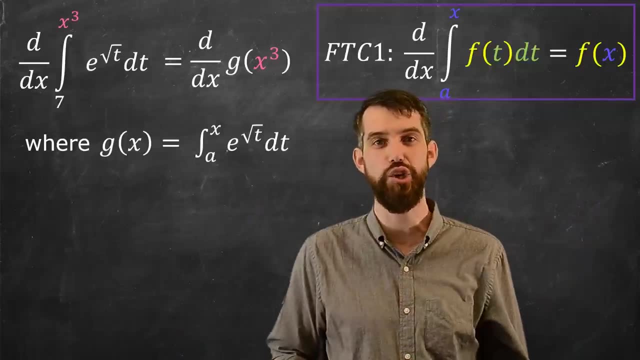 you put in an x cubed. Now why is that helpful? We know how to deal with g of x cubed. that's a simple chain rule. There's an outside function, g, there's an inside function, x cubed. We can do that by a. 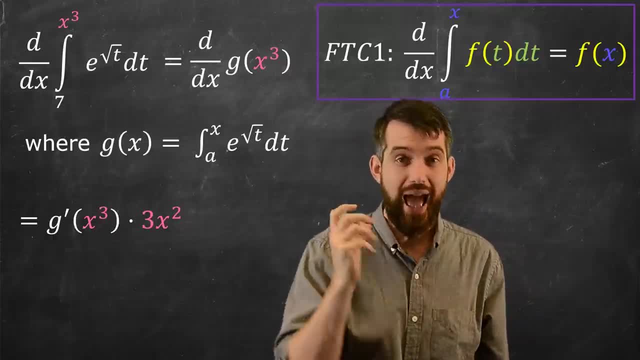 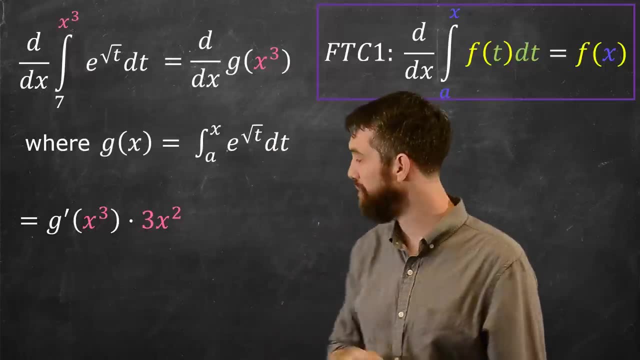 chain rule. so we say that we're going to do that by a chain rule and we're going to do that by a derivative of the outside function. at the inside function, the x cubed times derivative of the inside function. And then, final thing, how do I do g prime of x cubed? Well, the fundamental theorem. 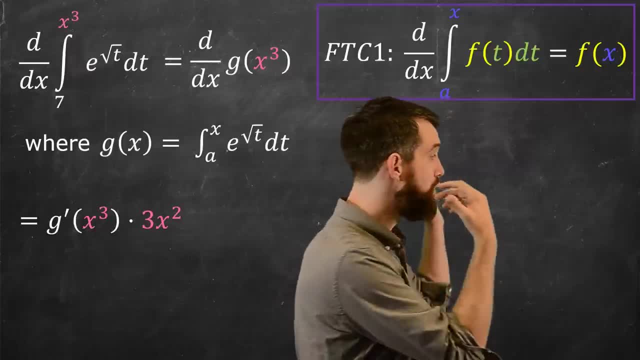 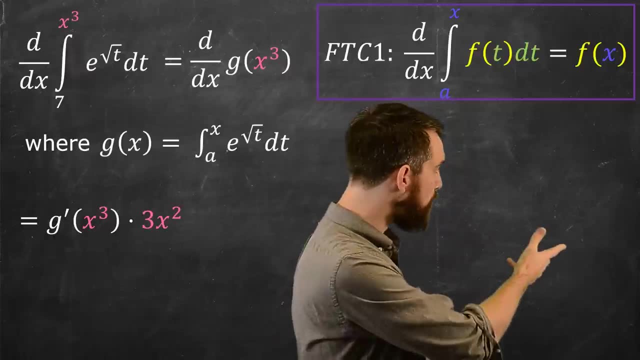 of calculus tells us what to do with the g prime. So let's just do whatever the g prime is, and we're going to evaluate that at x cubed. We're going to compose that with x cubed. So g prime is just the same thing as f by the fundamental theorem of calculus. So in this we go just to. 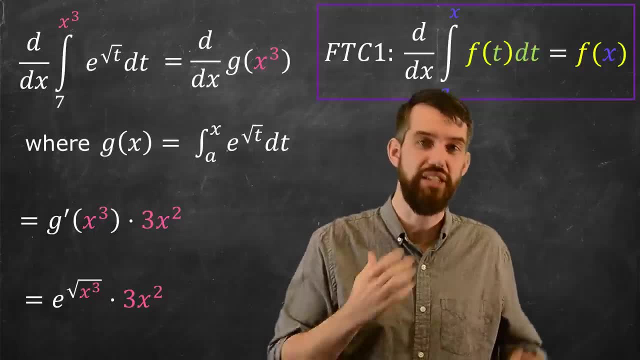 f of x cubed. So we're going to do that by a chain rule. and we're going to do that by a chain rule: f of x cubed. or in this case, the x is e to the square root. so e to the square root of x cubed. 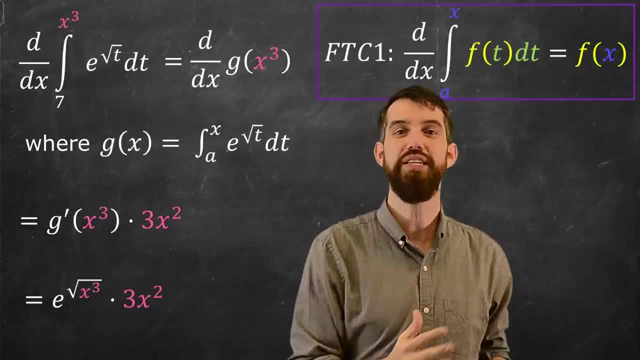 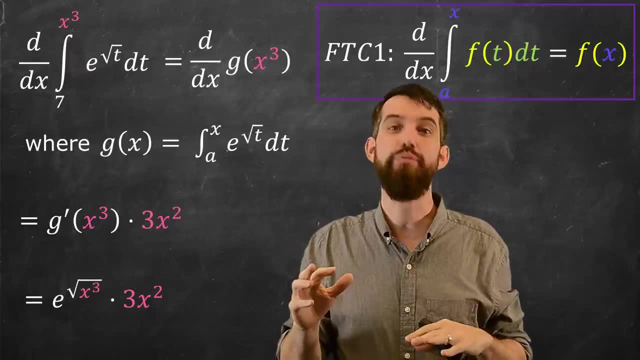 times 3x squared. So this was an example of how we could take something that sort of looked like the fundamental theorem of calculus applied to it, but not quite, and we managed to understand it as a composition and apply chain rule and apply the fundamental theorem of calculus and get that final value.